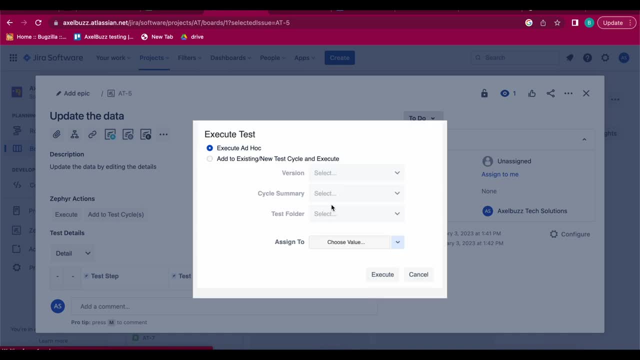 And then execute. Some execution window will get open. You can execute by two ways. execute Adoc: just in previous video I told you like without making any planning, just you pick up the test case and you simply execute that Any member can use this Adoc system and pick up the test case and execute. 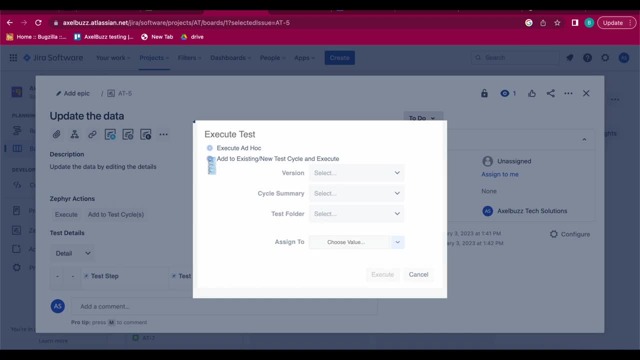 but if you are going through second method, which is this: add to existing new user or new test cycle and execute, then you can assign it to specific jira members, your testers or anybody, and then you can- that person only can execute the test case. so first, uh, we'll see by this ad hoc way, so choose. 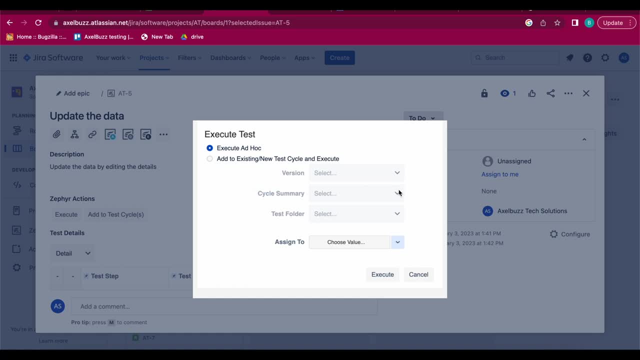 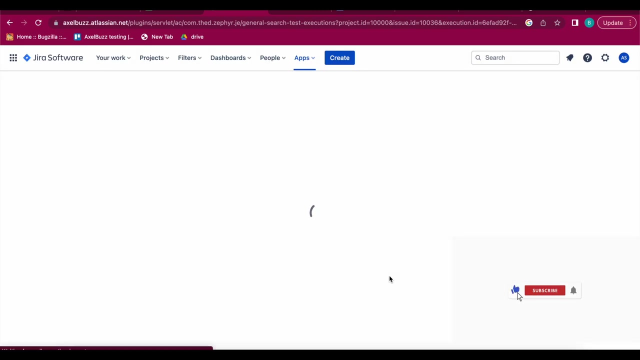 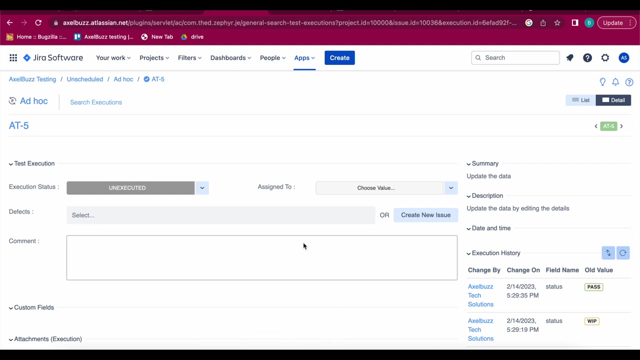 the version. so we will see this by executing in a dark way. after clicking on execution, this kind of window will get open. so, side by side, whatever is your test case, you perform that test and you come here here. if it is unexecuted means you have not yet executed. if your test case is pass, then you. 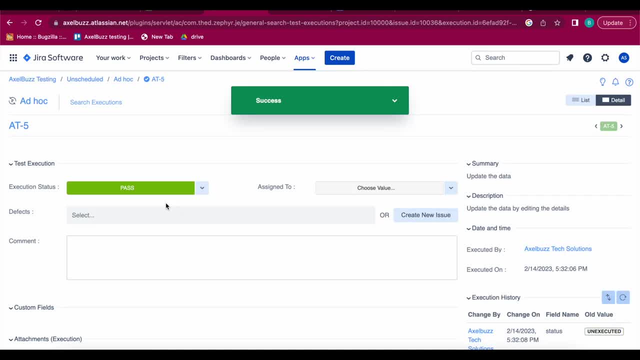 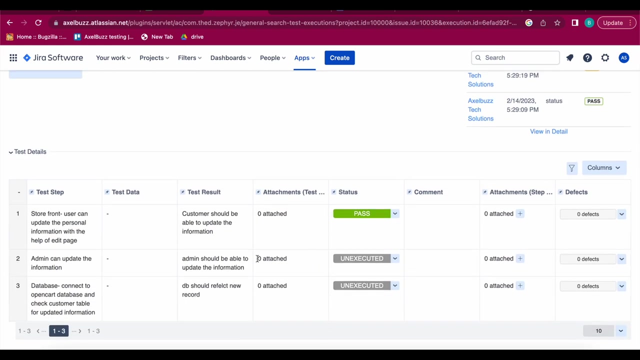 can select here: pass. if your test case is failed, you can select their fail. if you are working and it is taking time, then you can assign wip also, or somehow it is blocked. you are not getting any further if you go down. there are steps available so you can perform each and. 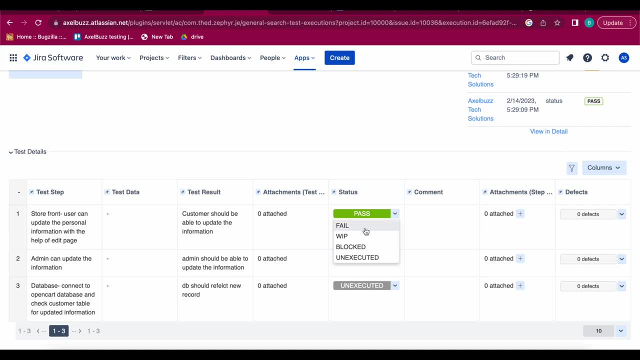 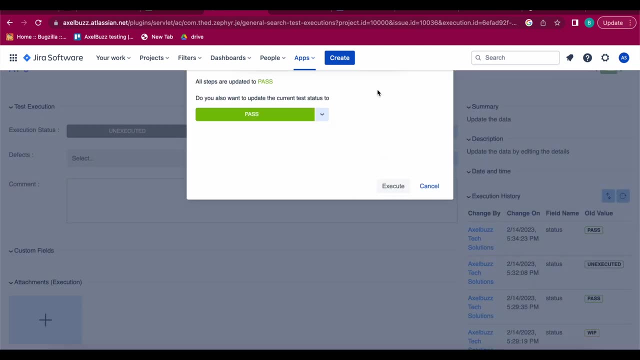 every step and then you can decide it whether it is pass or fail and you can mark it like that. so this is actually ideal way to perform the test case: perform each and every step, then automatically your test will go cover. so something, some message like this will come: all the steps are pass, so your test. 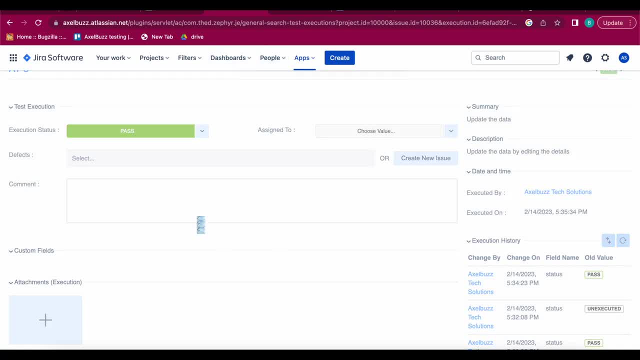 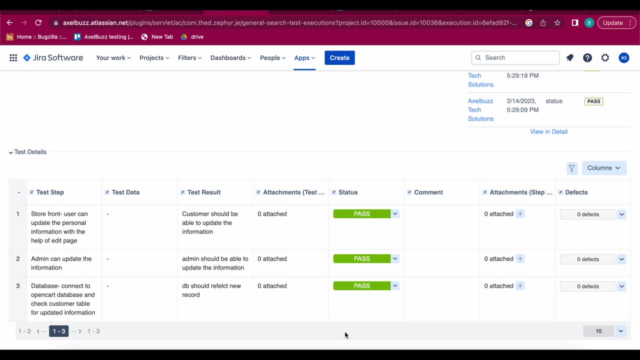 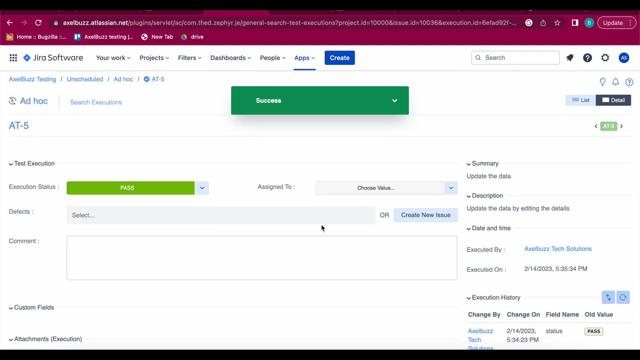 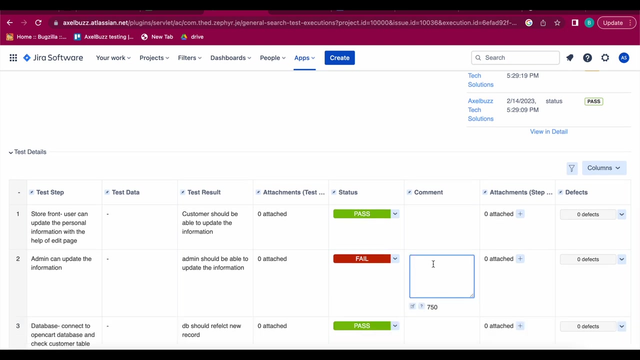 case will turn pass automatically. if your all test steps are pass automatically, your test case will perform automatically. your test case will mark it as passed. but if anything fails, then it will mark your test case will go as fail. you can write down why it is fail or you can comment. if any, then if 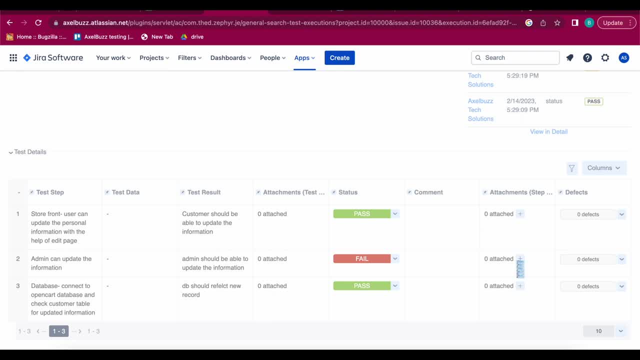 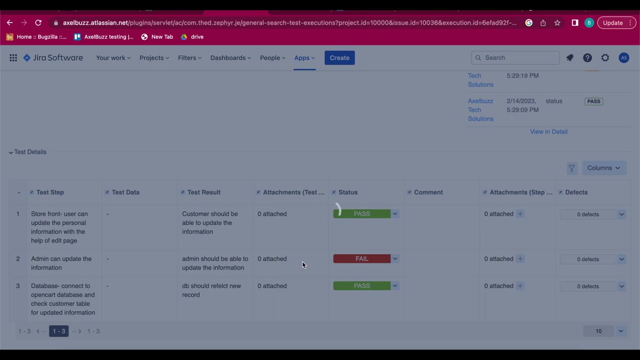 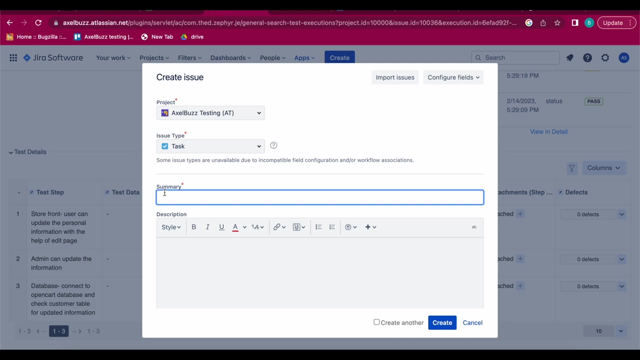 you have any attachments in these screenshots where the defect is, then you can attach here and simultaneously you can raise the bug and link this with your failed test case. so add defect, create defect and then one new create window will get open. so if you click on add defect, then one new create issue. 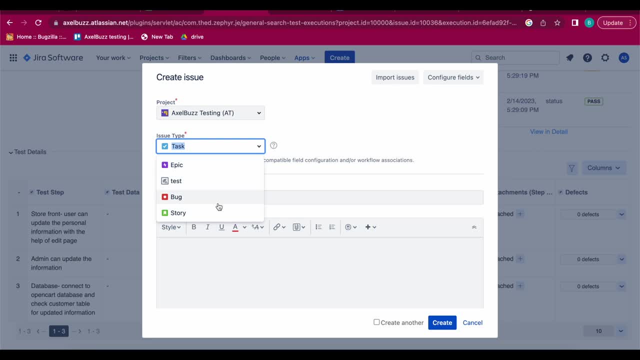 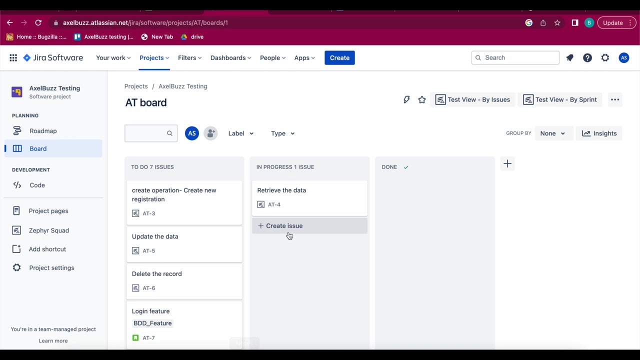 window will get open then here you can choose as a bug and then you can log this defect. why that test case? how that test case got failed and you can create it. if you create, that is automatically linked with your test case- was first way, how to execute the test case. now I'll show you another way. let's go to Zephyr. 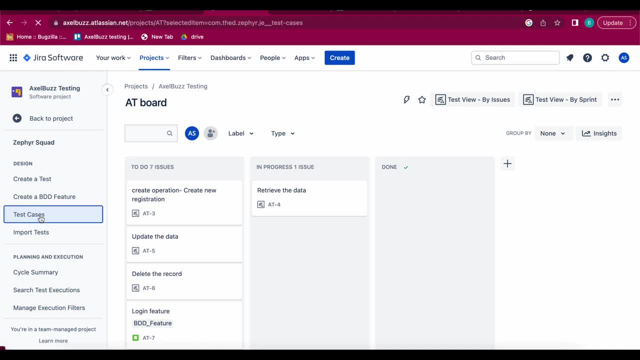 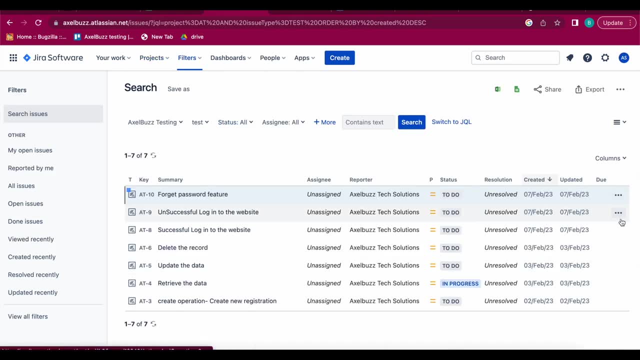 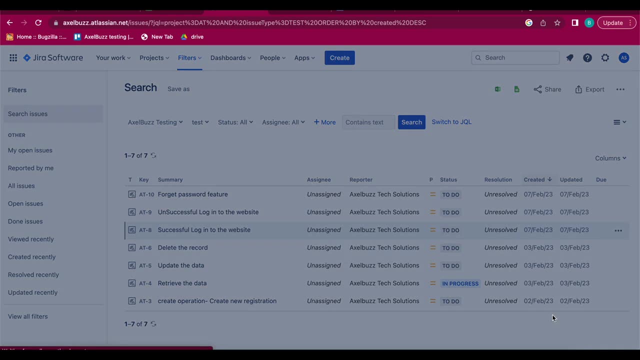 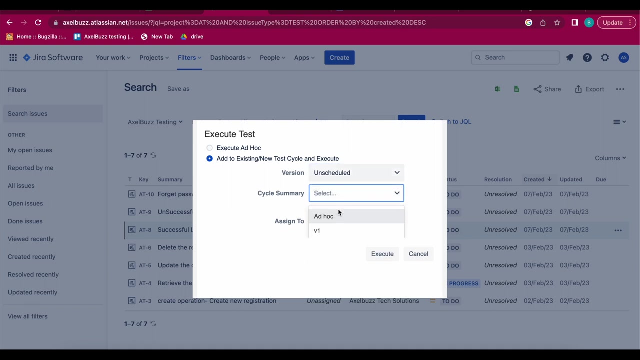 squad. then your test cases. go to advanced search. here you will see execute. same kind of window will get open. you can add unscheduled version version v1, this folder, regression. suppose I want to add this test case in regression folder, then execute. then it will get added to your regression folder and execution. 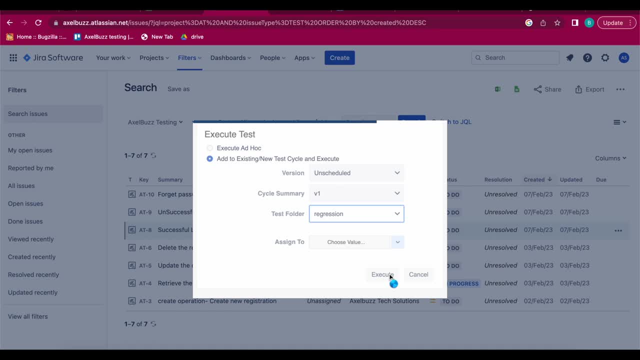 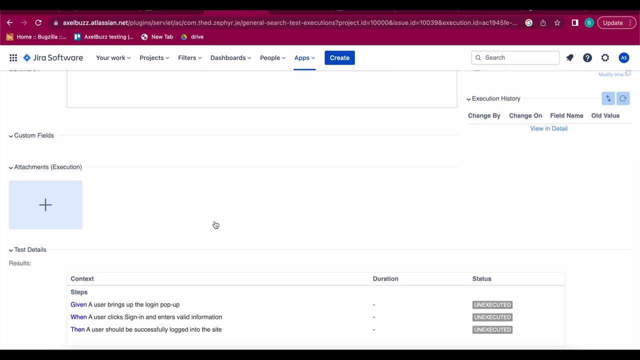 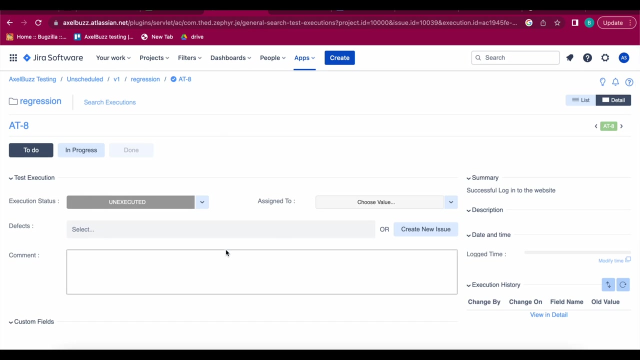 window will get open and goals will be labeled and running the testlemme, and and and same execution window will get open and then the rest rest of the procedure will be same. so you can, if you are, if your test case is already passed, you know it. then you can simply execute. 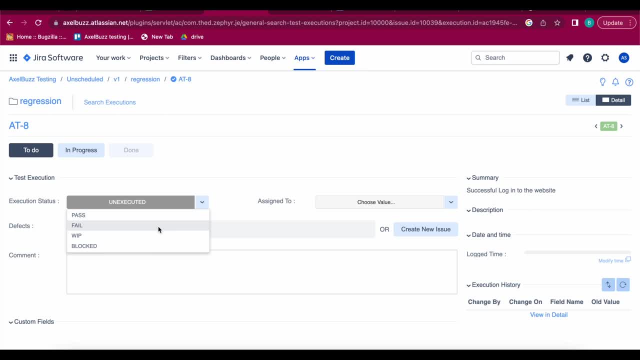 unexecuted. you can change it as pass or fail, or if you know your test cases fail or you, then you can simply fail from here and then you can create new issue or you can link. if issue is already present, you can link from here or you can create new issue. same: create issue window will get open, then you. 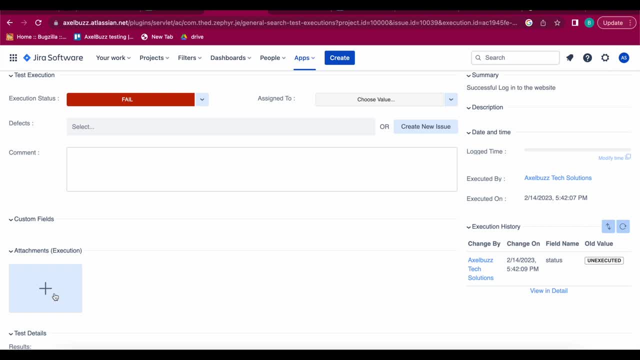 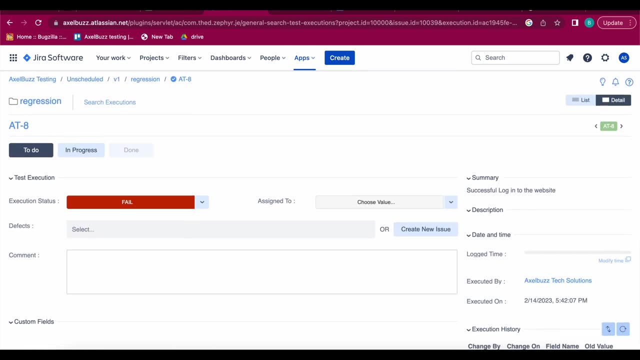 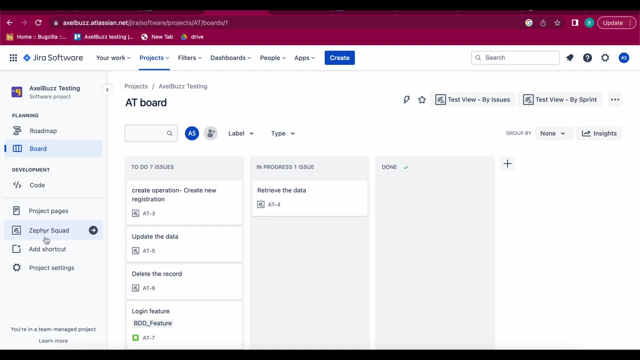 then you can attach screenshots or any document if you want to use to link with defect, then you can attach it from here. rest of the process will be the same. so there is one more way to execute the test cases. let's go to zephyr squad, then test summary. 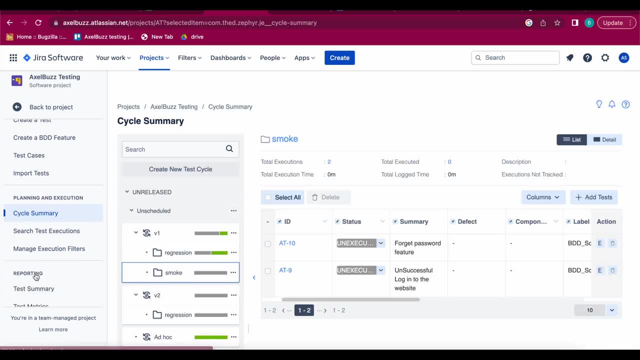 in cycle summary. then in cycle summary, we have created a cycles and version according to their versions, and folders according to their types of test cases. so you can simply do that. you can open this folder. whatever test cases you have to execute, just pick up the folder and execute. 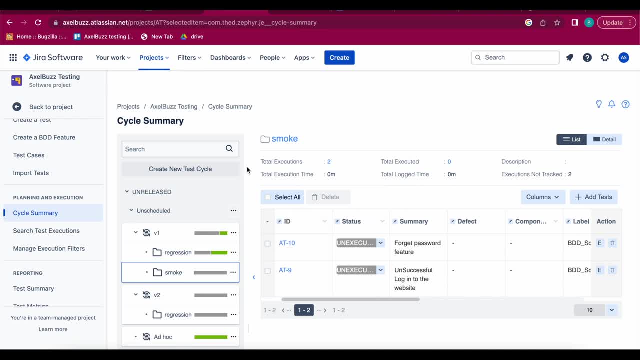 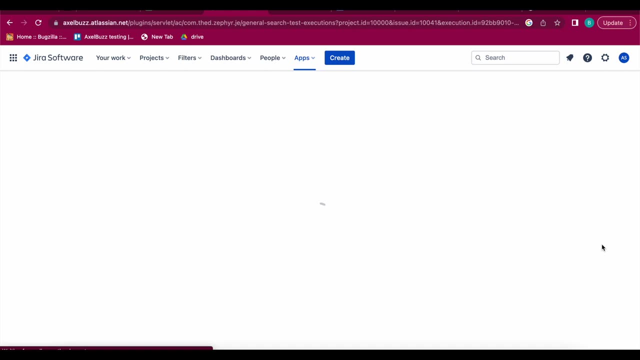 all the test cases here. i have opened smoke test case folder, so let's see there are two test cases available in my smoke test case folder. so click here in action. you'll see this. e capital e just click on there and then same execution window will get open. 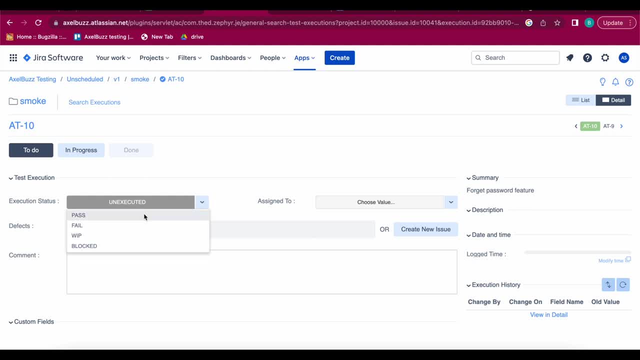 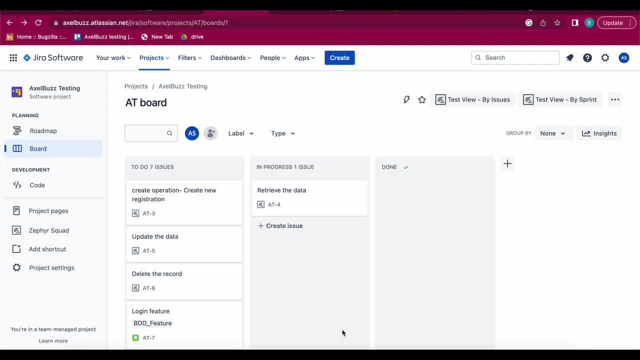 and you can execute the test case and change the status as pass or fail. now you have executed few test cases and you are not able to remember which test cases you have executed and which are left. so let's see how you can check out that. so let's go to zephyr squad. 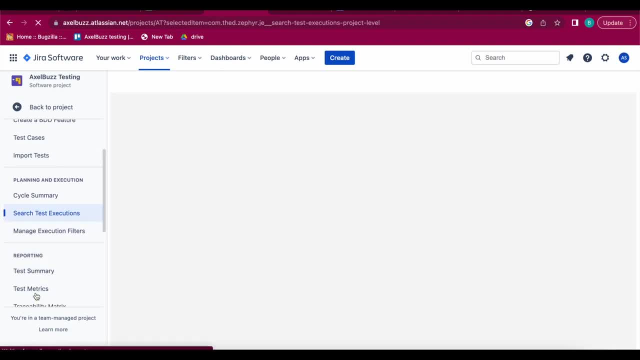 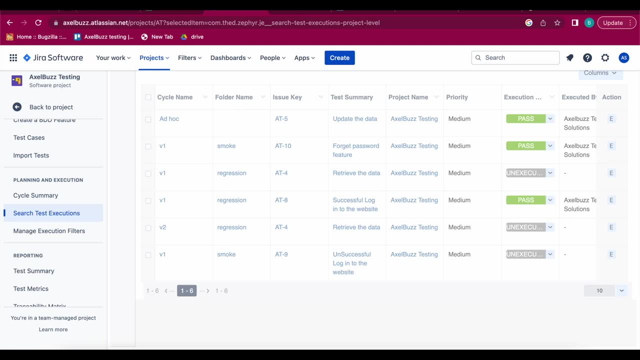 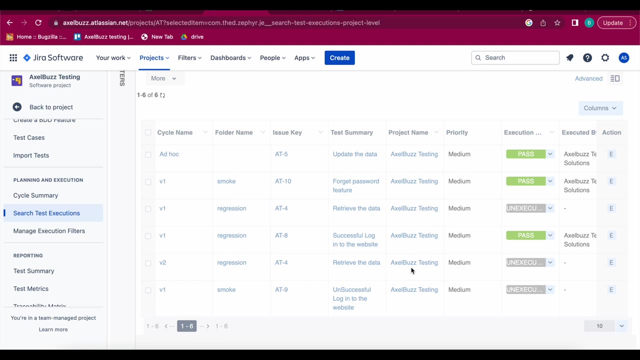 and search test execution. this tab will give you all the test summary: which test cases are executed, which are passed, which are failed. so from here, directly, which which? whichever test cases are not executed, you, from here, only you, can check out that and whichever test cases are left. so if your test case is executed, what are you going? 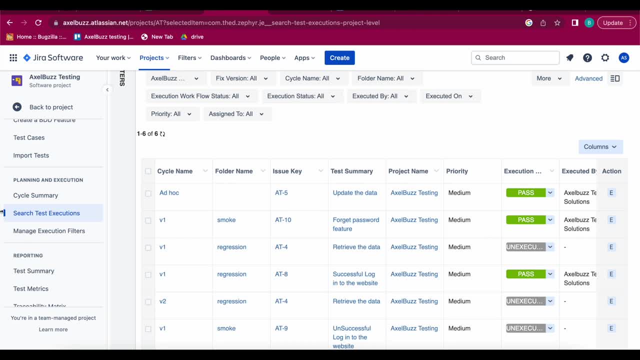 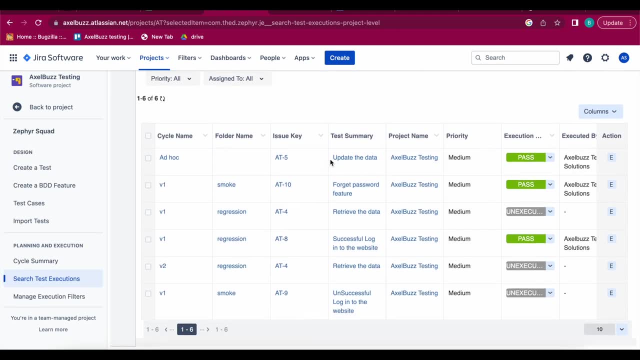 to do this will be something like check the test case manual. you can also find all the test cases happening. for example, if i want test case to be free, will i click test case and i go to test caseette. poi, at test case for this, you will notice all the test cases are accepted. 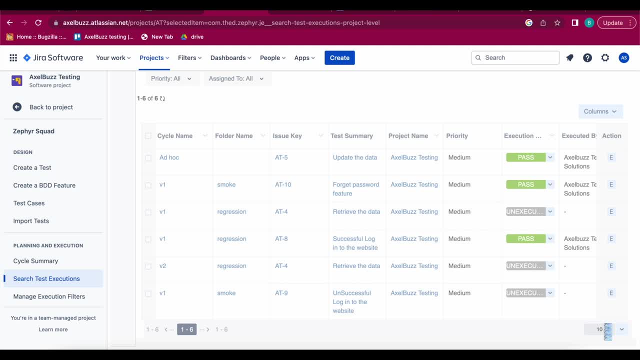 we see all the test cases in the test case study are empty. so when you see these types of test cases, try to Megan. all my test cases are really good. as you can see, when i clearly enter these, there are about five or so test cases are left. 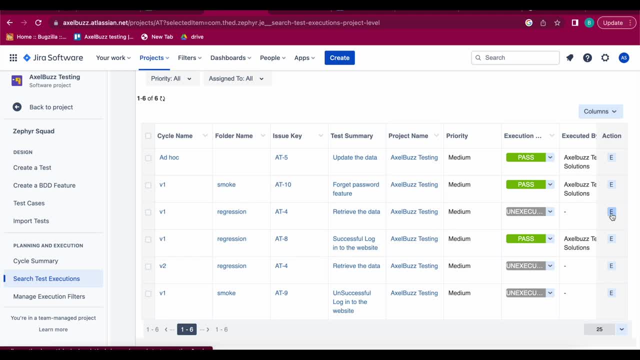 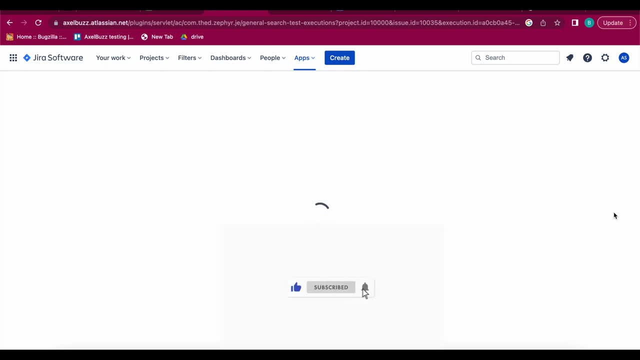 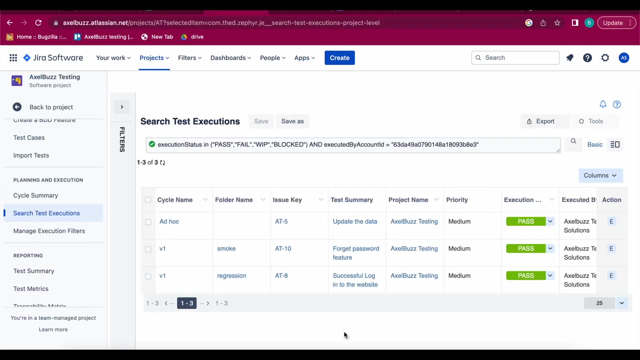 are left behind. you can simply directly go click on this action E and directly execute this test case from here itself. same execution window will get open. same execution window will get open here and you can execute your test case. there are filters. also, you can check out my executed test, my fail executions, my un-executed test and you. 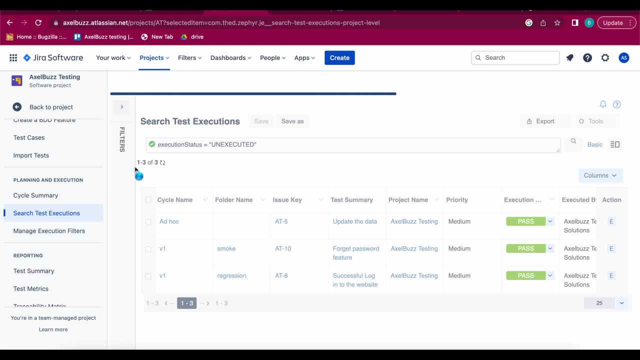 will. you will get direct list. whichever test cases are fall under that filter. so so, so like this: if you click on un-executed, all un-executed test cases will come. these are few ways how you will execute test cases in zephyr, how you will mark them as. 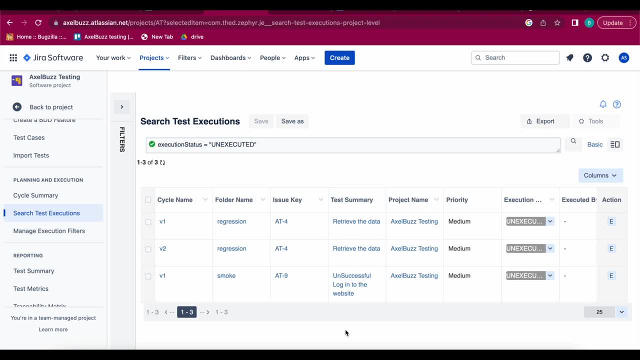 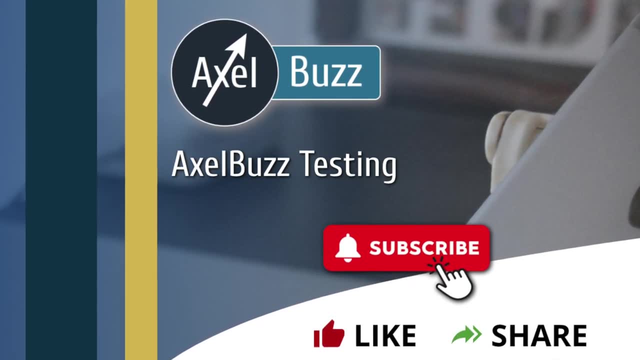 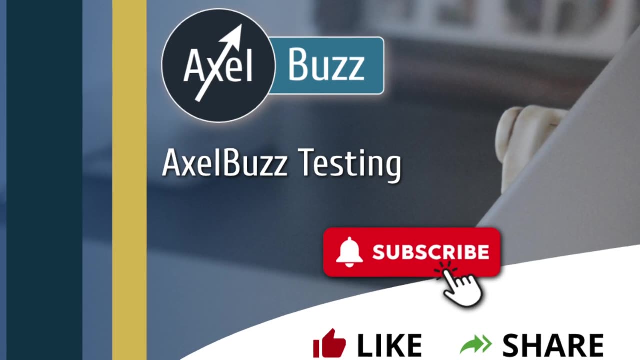 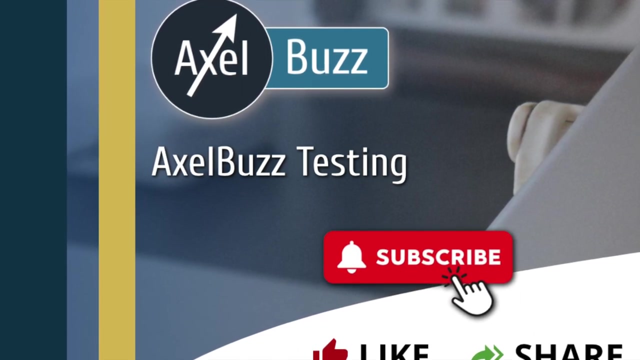 pass or fail or any other, and this is it for today. hope you like this video. if you like this video, please hit the like button and subscribe to our channel, if you haven't yet. we post videos on every tuesday and friday. if you have any queries or any suggestions, please comment down to us. so until then, happy testing. bye, bye.